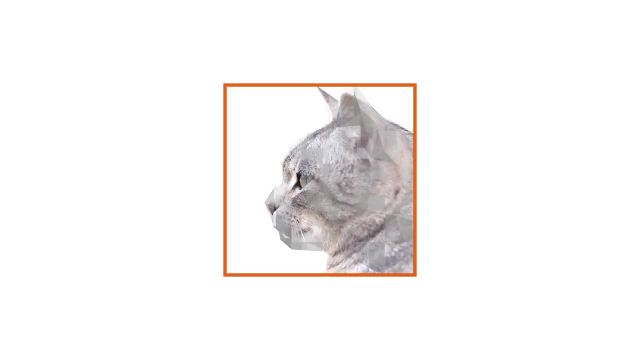 that happens here. Subtitles by the Amaraorg community. Think of it this way: An image is complex. A convolutional neural network simplifies it, so it can be better processed and understood. Let's look now at what's inside a convolutional neural network. 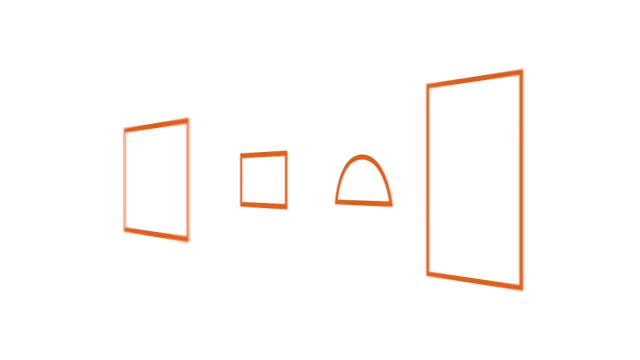 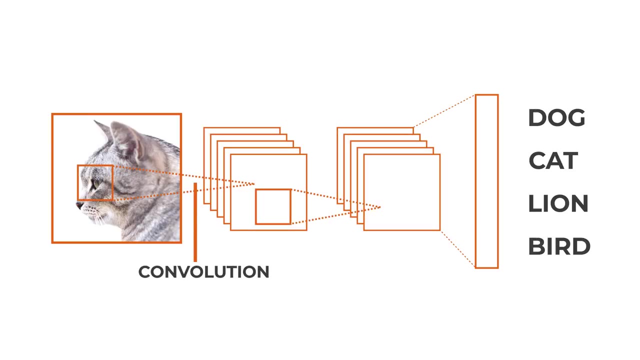 Like a normal neural network, a convolutional neural network is made up of multiple layers. There are a couple of layers that make it unique: The convolutional layer and the pooling layer. However, like other neural networks, it will also have a ReLU or rectified linear unit layer and a fully connected layer. 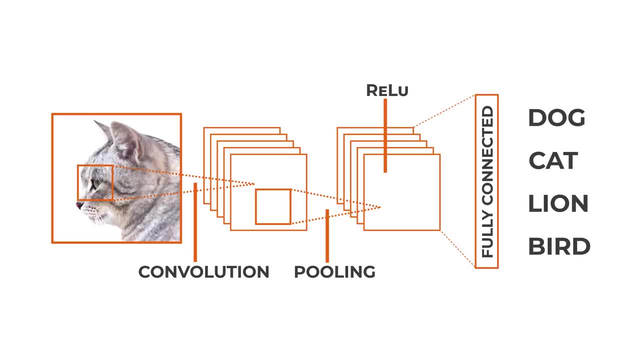 The ReLU layer acts as an activation function, ensuring non-linearity as the data moves through each layer in the network. Without it, the data being fed into each layer would lose the dimensionality that we want to maintain. The fully connected layer, meanwhile, allows you to perform classification on your dataset. 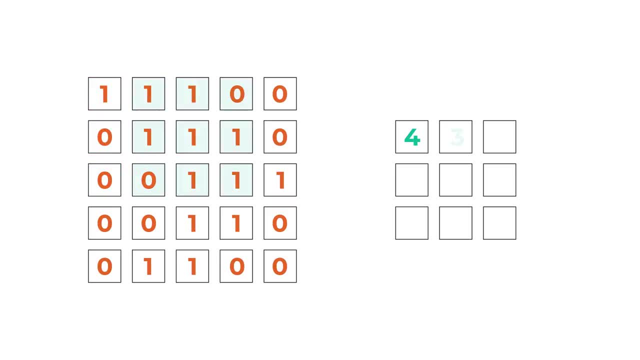 The convolutional layer is the most important, so let's start there. It works by placing a filter over an array of image pixels. This then creates what's called a convolved feature map. It's a bit like looking at an image through a window which allows you to see specific features you might not otherwise be able to see. 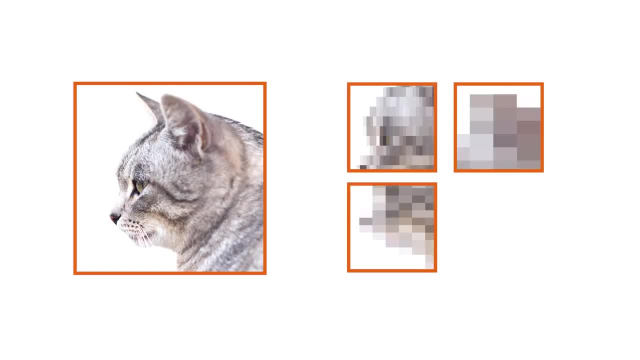 Next we have the pooling layer. This downsamples or reduces the sample size of a particular feature map. This also makes processing easier. The pooling layer allows you to process much faster, as it reduces the number of parameters the network needs to process. 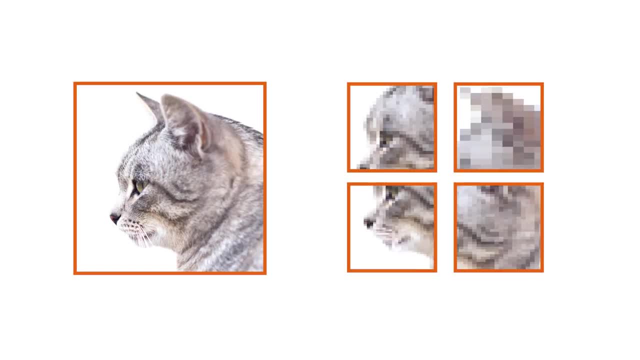 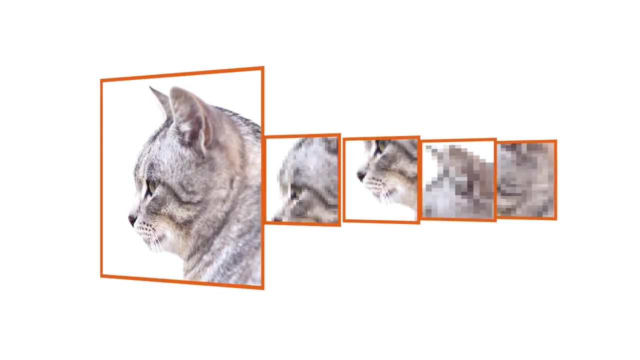 The output of this is a pooled feature map. There are two ways of doing this: Max pooling, which takes the maximum input of a particular convolved feature, or average pooling, which simply takes the average. These steps amount to feature extraction, whereby the network builds up a picture of the image data according to its own mathematical rules. 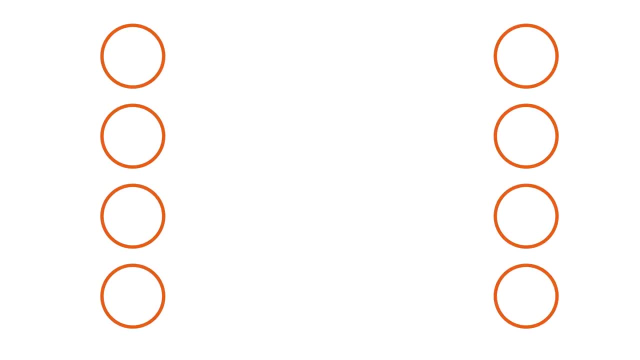 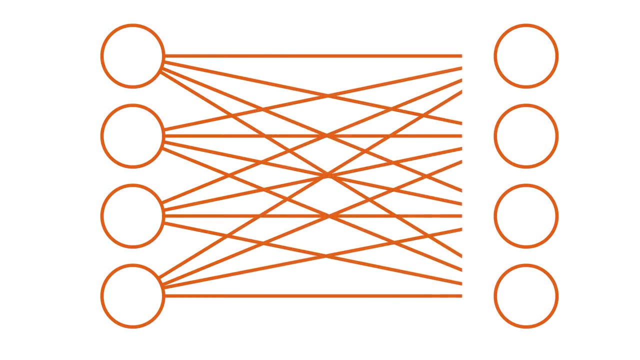 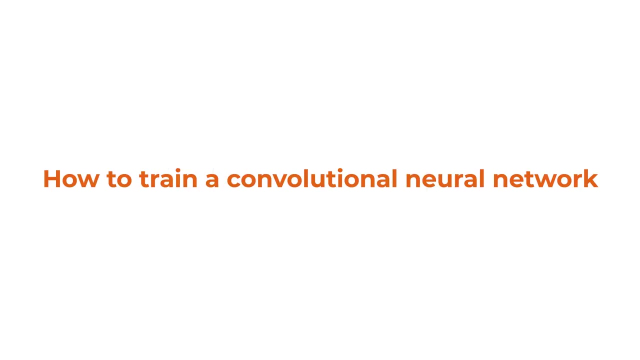 If you want to perform classification, you'll need to move into the fully connected layer. To do this, you'll need to flatten things out. Remember: a neural network with a more complex set of connections can only process linear data. There are a number of ways you can train a convolutional neural network. 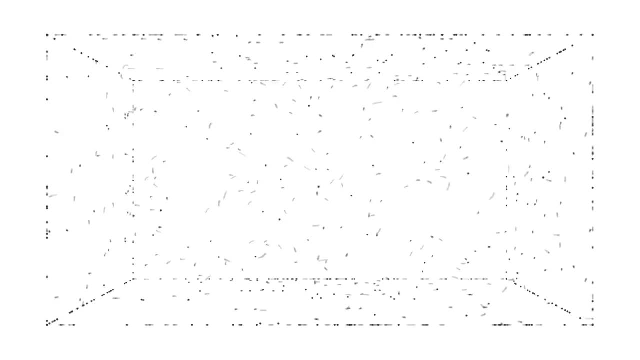 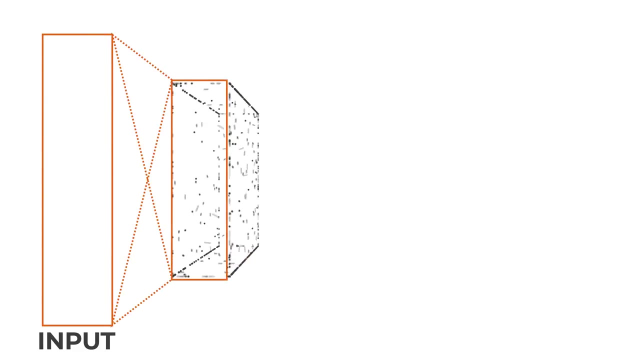 If you're working with unlabeled data, you can use unsupervised learning methods. One of the best popular ways of doing this is using autoencoders. This allows you to squeeze data in a space with low dimensions, performing calculations in the first part of the convolutional neural network.